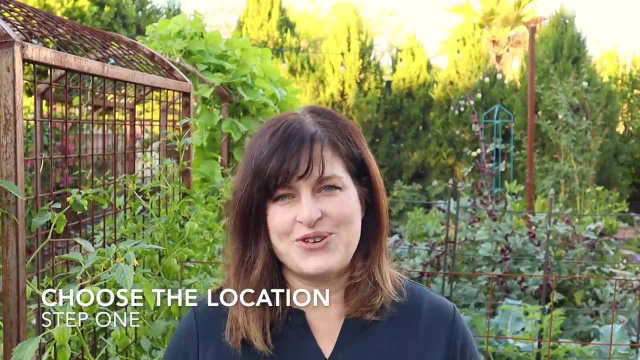 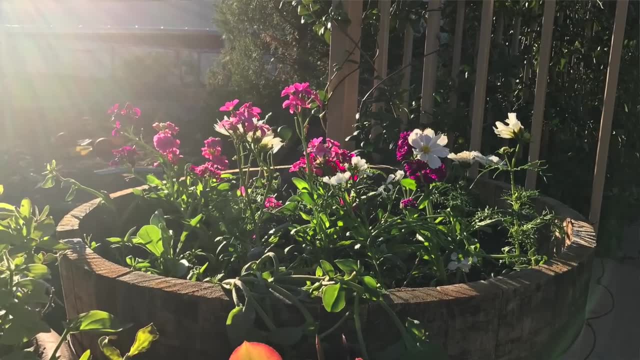 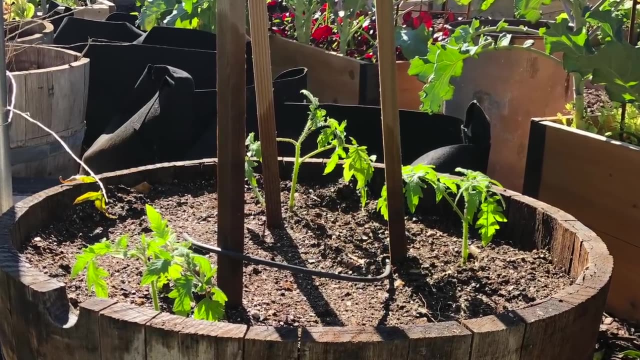 soil and get growing. The first step is to choose the location for your container garden. The most important thing to remember is that we can't grow anything without sunlight. Pay attention to how much sunlight that area receives. Ideally, it gets at least six to eight hours of sunlight each day. 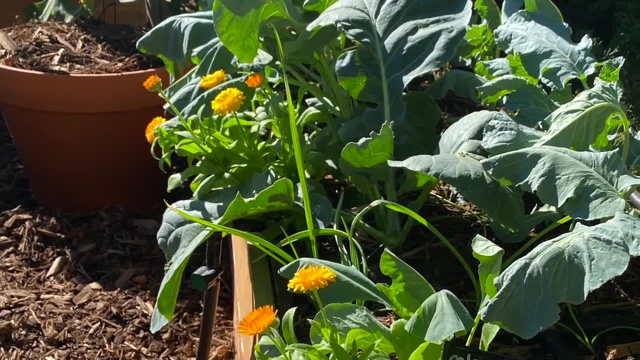 If you have a choice, choose an area that receives morning sun. Hopefully there's easy access to water and that is very Portland. If there is no improvement in access in the summer, then a lot of wind is hard to follow or pretty clear water might continue getting wet Again. if you are. 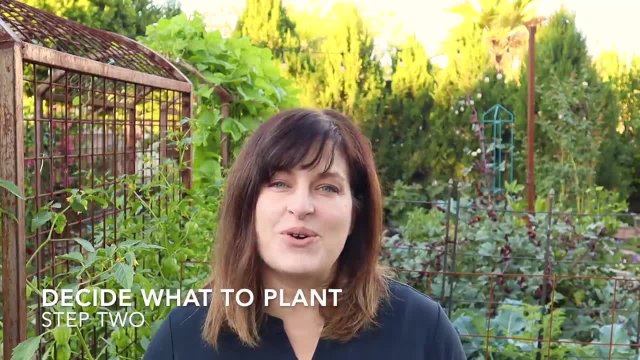 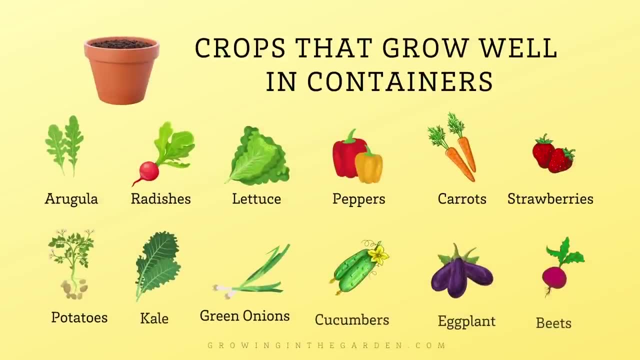 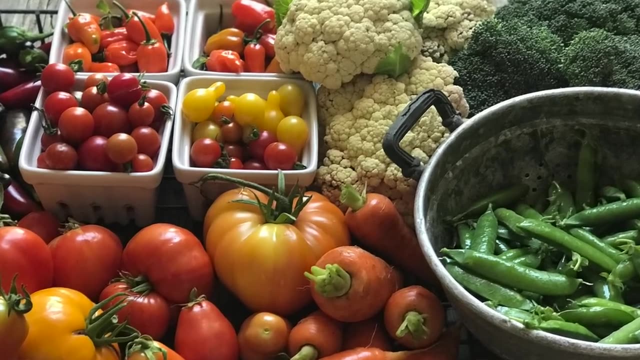 mostly not able toад up picking holes. the sun will step on your plant by ajig When it cheesecake for Nike or in that location as well. The next step is to decide what you're going to plant. Make a list of things you would like to grow. Start with things you like to eat. 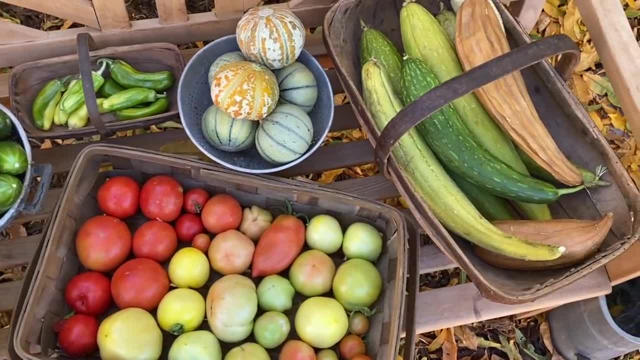 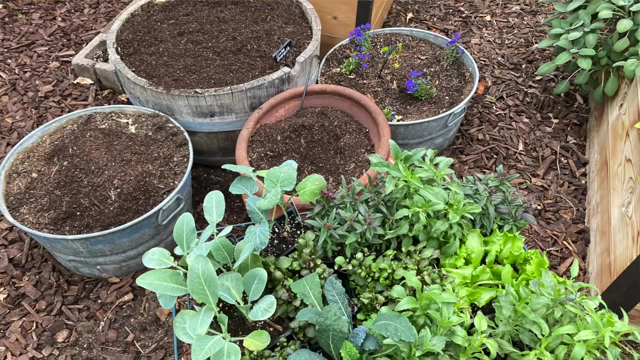 Maybe try a few new things too. Once you have your list of things you'd like to grow, find a planting guide for your area. Look at the planting guide and find out what can be planted right now. Evaluate the space you have available. Make sure. 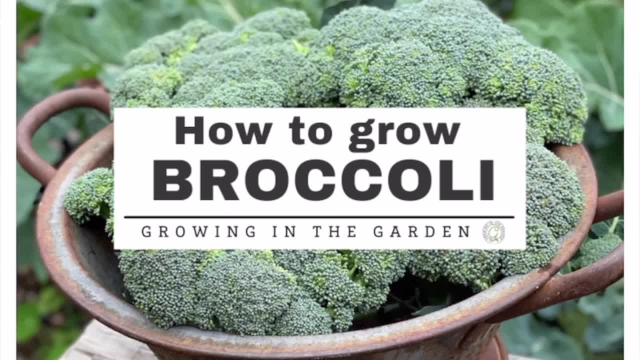 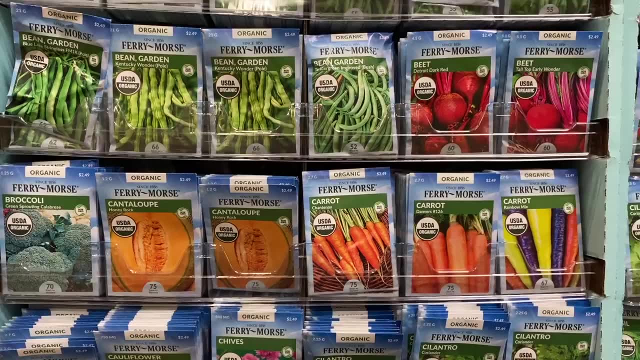 you have enough room to grow the selected plants. Take time to learn about each of the plants you'd like to grow and find out if it needs to be planted from seed or transplants. Head to your local nursery or favorite online retailer and pick up those seeds and transplants. The next step is to choose. 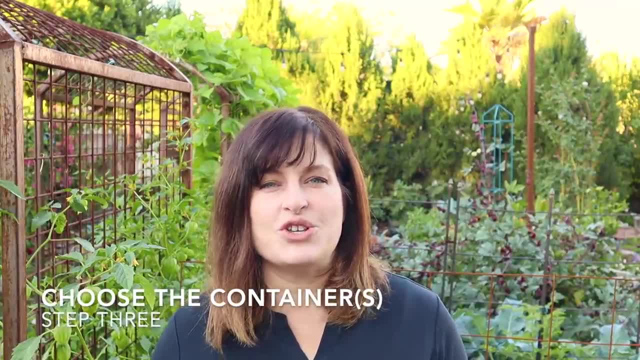 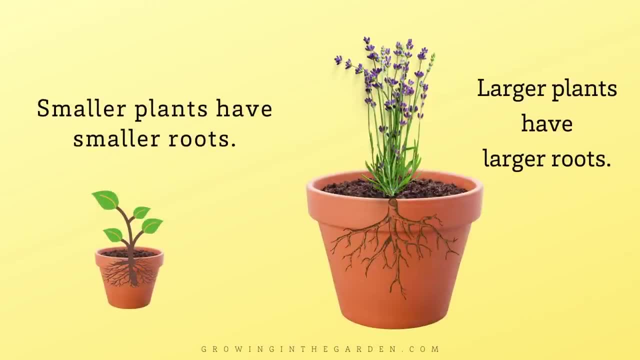 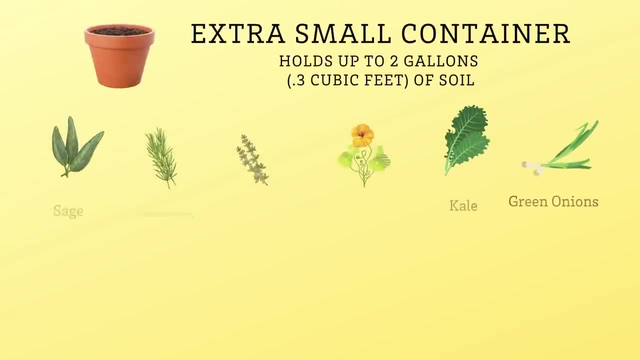 your container, and there are two important things to consider when choosing your container. The size of a plant is limited by how large the container is. It's important to grow the right plant in the right size pot. Here are a few guidelines for what size pots different plants need. 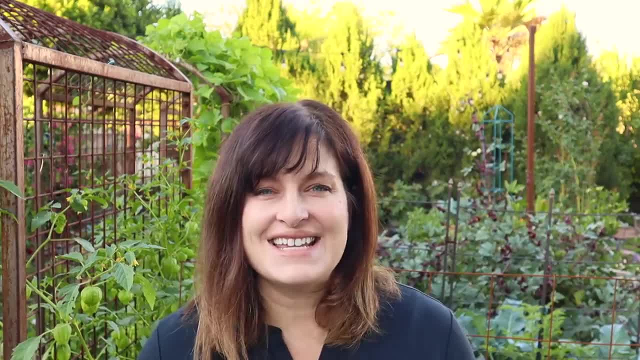 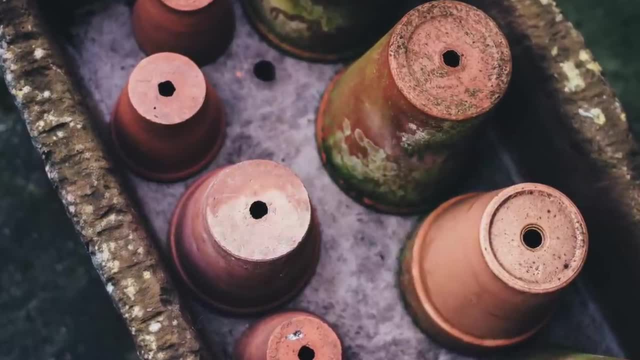 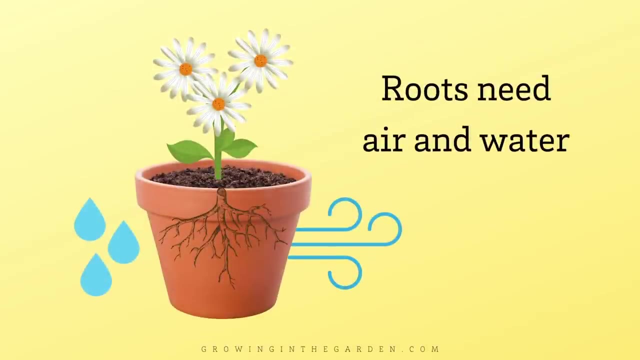 Also make sure your container is filled with good drainage holes. The next thing to consider for your container is to make sure that they have drainage holes. The hole allows excess water to drain out of the container. Roots need air as well as water in order to breathe. Too much water will suffocate. 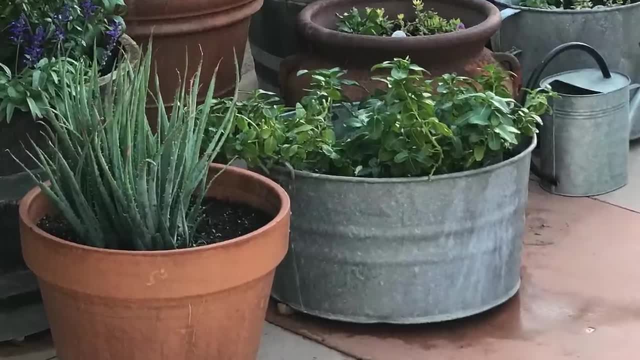 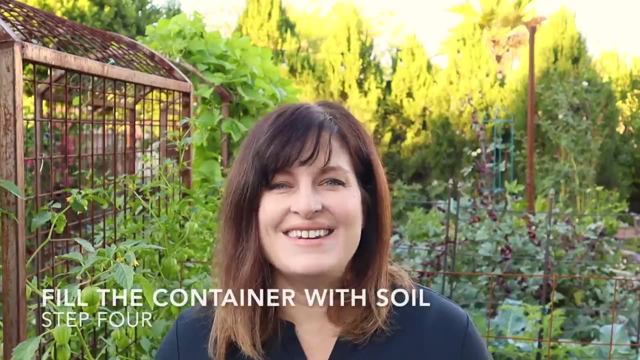 and drown those roots. If the container you're growing on is on a hard surface, lift that container up with pot feet. If your container is on soil or grass, that seep out, no problem. the next step for container gardening is to fill that container with soil. 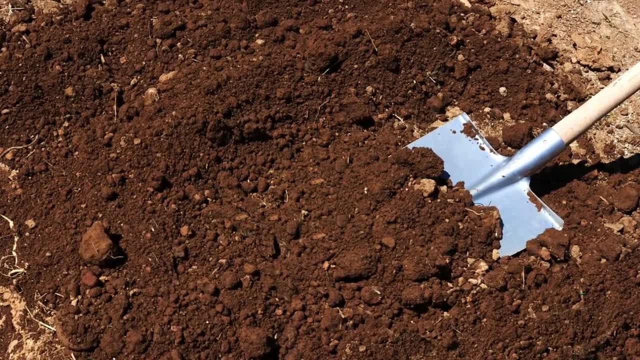 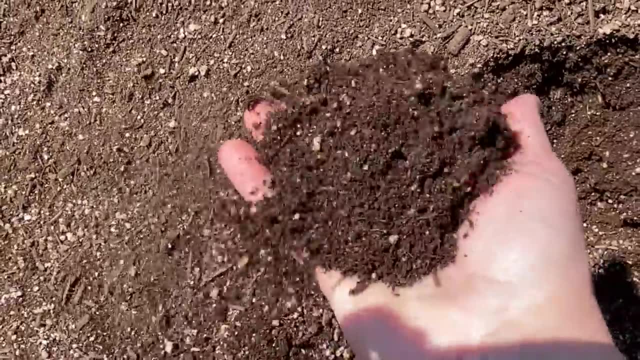 regular soil is too heavy for containers and doesn't provide the roots the air and water that they need to grow well. look for a quality raised bed mix or potting soil. it should be light, fluffy and drain well. look for a combination of compost, coconut, coir and vermiculite or perlite. 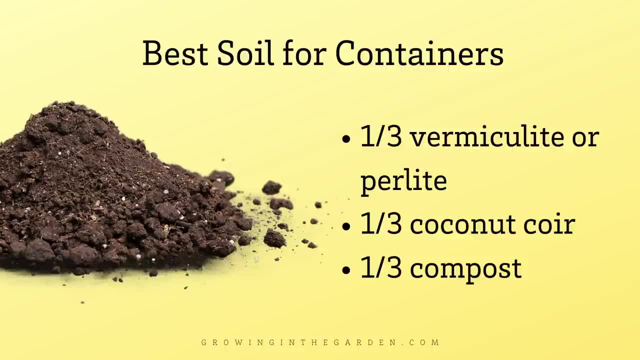 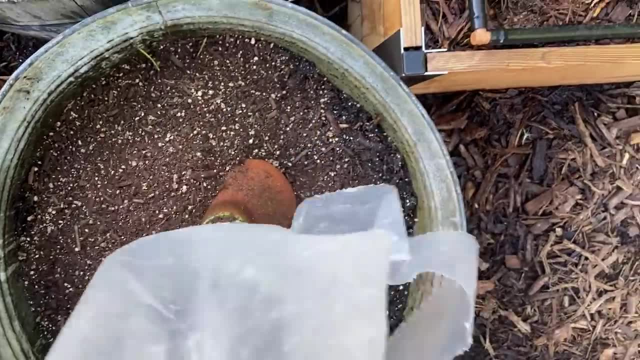 the right mixture of ingredients provides nutrients, air and water for the roots and gives your plants the best chance for success. put your pots in place and fill them all the way up with soil. you don't need to add any filler to the bottom. the more soil, nutrients and water available. 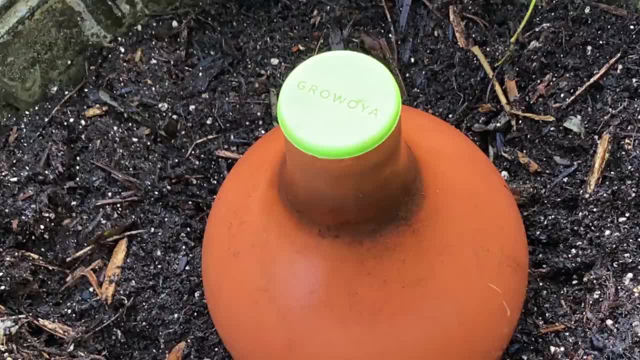 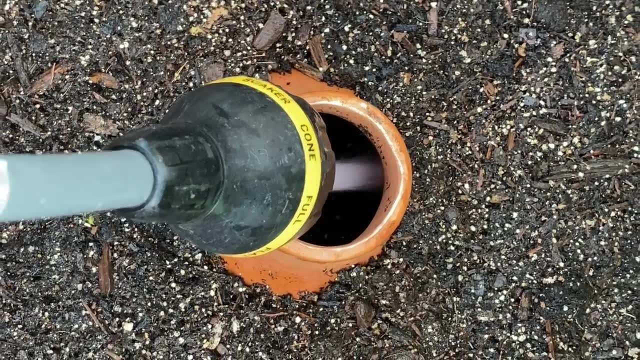 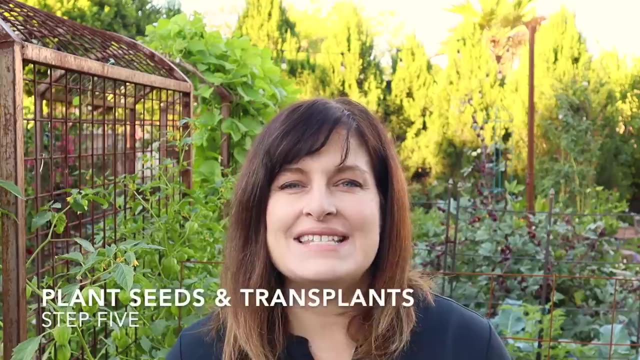 to your plants, the better. if you're going to add an oya to your container, now is the time to do it. an oya is a clay vessel that is buried underground and filled with water. that water gradually seeps out as needed by the roots. oyas are by far my favorite way to water containers. the next step: 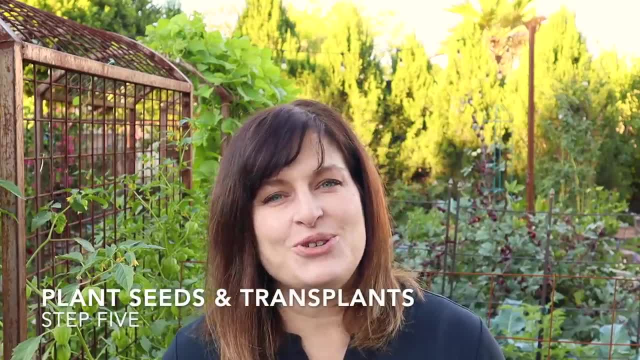 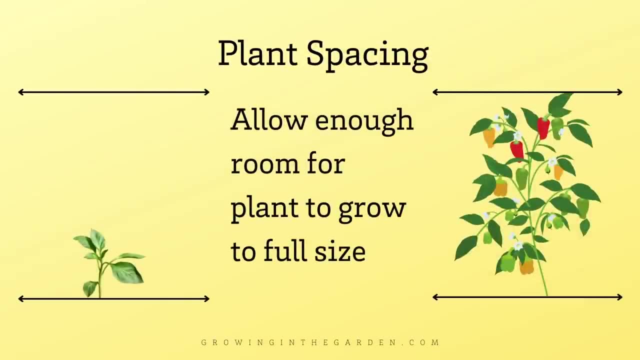 is to plant your seeds and transplants and your containers. as you do this, there are three things to keep in mind. the first thing is spacing. adequate spacing is crucial for growing plants. plants that are too close together often crowd each other out and compete for sunlight, available nutrients, and often lead to pests and 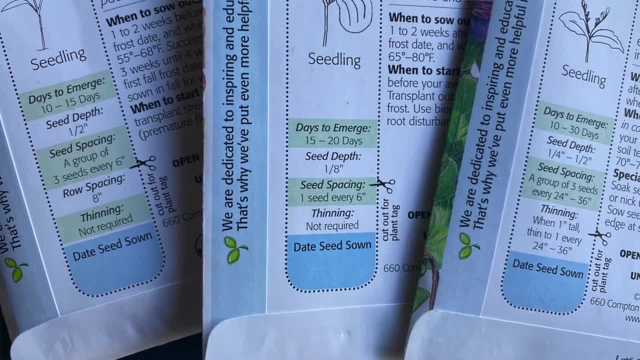 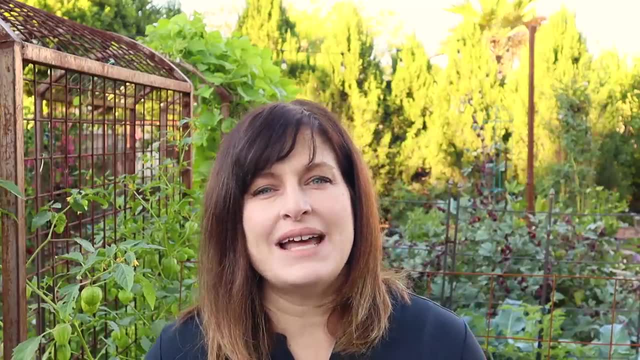 diseases. use the spacing guidelines on the backs of seed packets or on your transplants as a guide to give your plants enough room. when planting transplants, it's important to plant them at the same level of the nursery pot. Carefully remove that plant from the pot. dig a hole. the same depth. 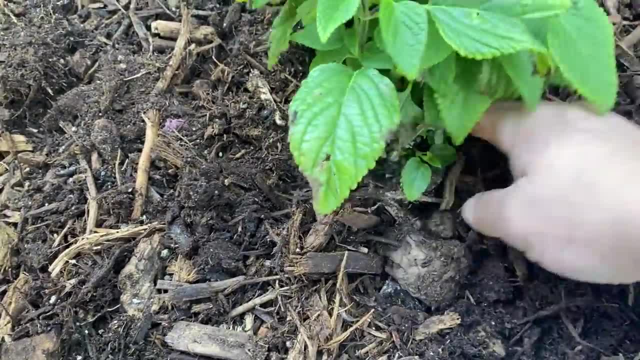 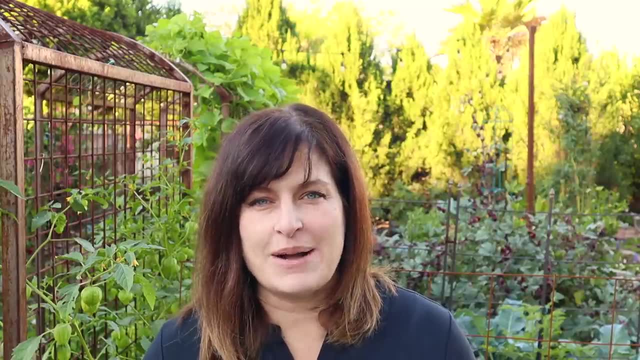 and put it in right at the same level. An exception to this would be plants like tomatoes. They're often buried much deeper and roots will grow along that stem. When you're planting seeds, there are a couple of things to keep in mind. Typically, plant the seed two times the depth Once you start. 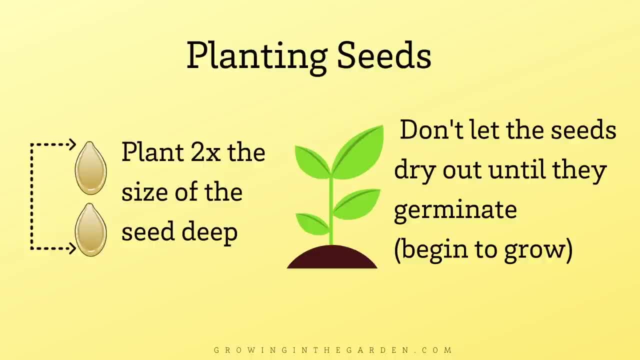 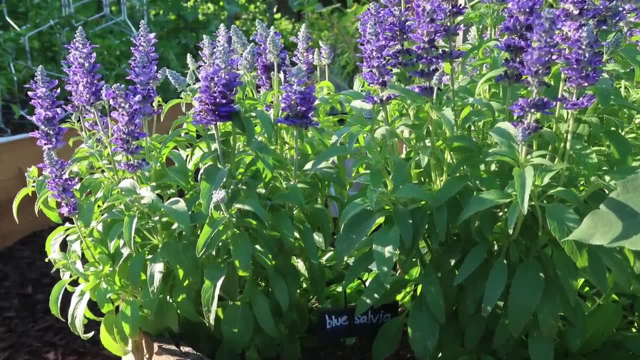 watering seeds. it's important to keep watering them until they germinate. Let's talk for a minute about watering your containers. When plants are grown in containers, the plant's roots can't seek out water like they can if they're grown in the ground. Plants are dependent upon. 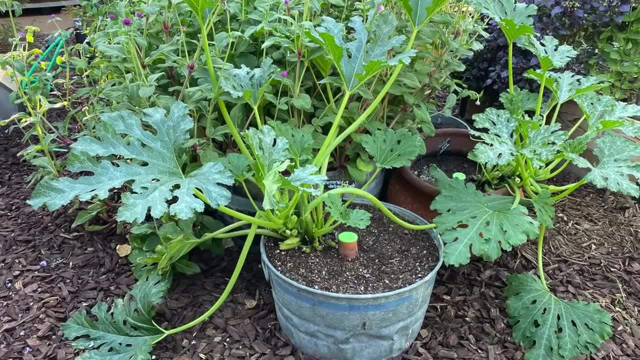 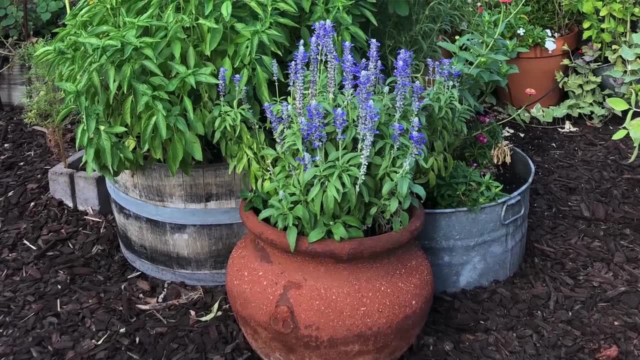 you for water. Many problems in the garden can be traced back to incorrect watering, Either too much water or not enough water. When you first plant seeds or transplant, they're going to need watered a little bit more often until those seeds germinate and those transplants get established. 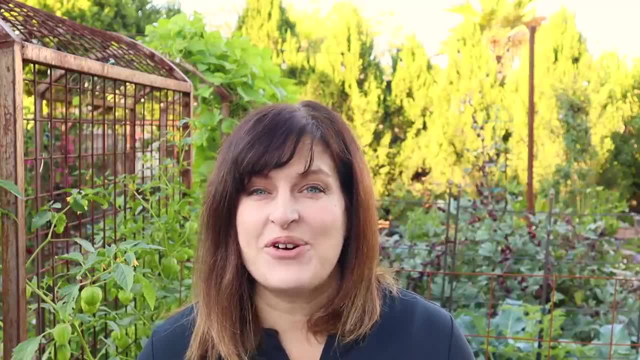 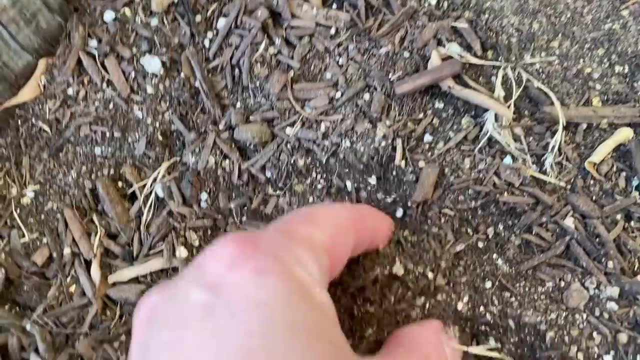 How often should you water your containers? The answer is: however often they need water. So how do you know if they need watering? The best way to tell is to pull back the mulch and stick your finger in about an inch or so and see if it is dry, If 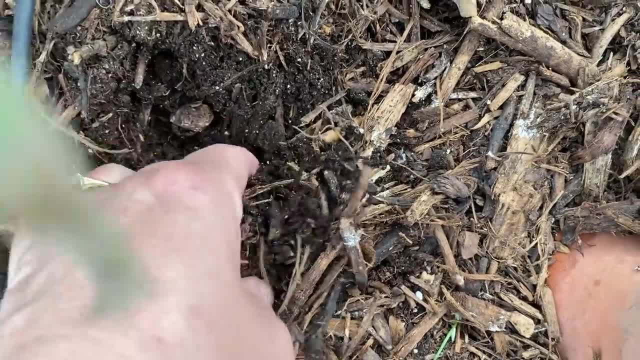 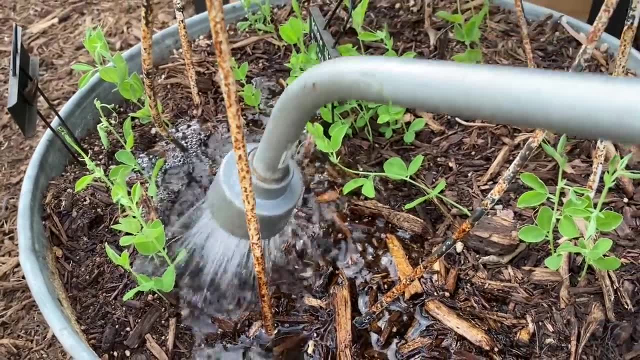 it's dry, it needs water. If it's still moist, then they don't need water. Droopy, wilted leaves are a sign that you waited too long to water. When you're watering, be careful to water the soil, not the plant. The plant's roots absorb the water in the soil and then the roots then pass that water. up through the stem. When you're watering, the soil and the roots absorb the water in the soil and then the roots then pass that water up through the stem. When you're watering, be careful to water the soil and the roots then pass that water up through the stem and into the leaves. 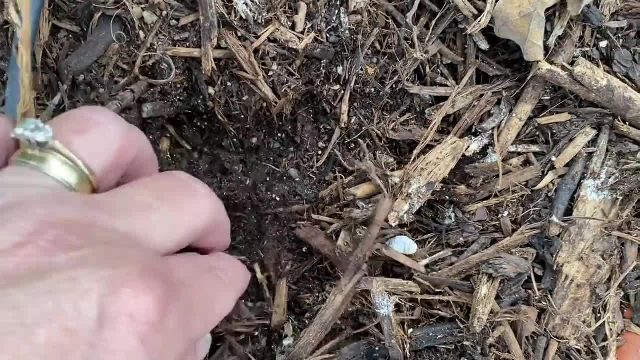 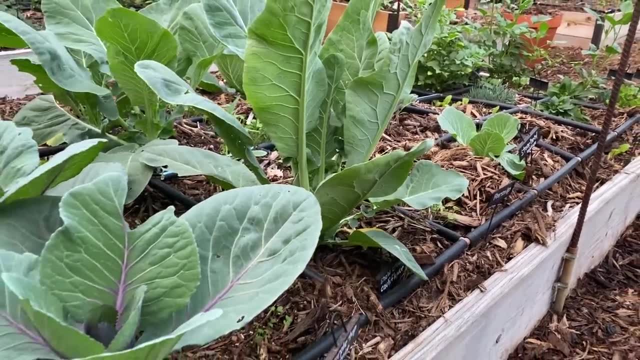 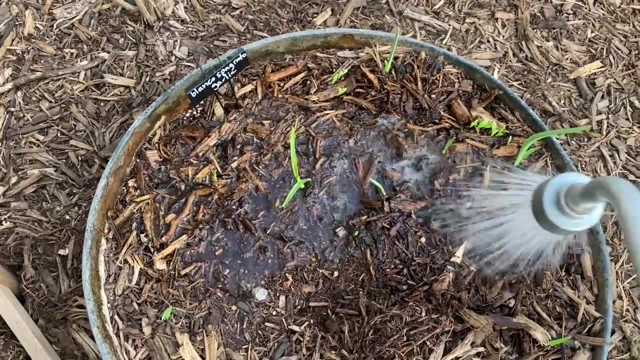 Adding a one to two inch layer of mulch in your containers helps slow evaporation and keeps that moisture in the container. Plants grown in containers will often need to be watered more often than plants grown in raised beds or in the ground. I like to use a shower attachment. 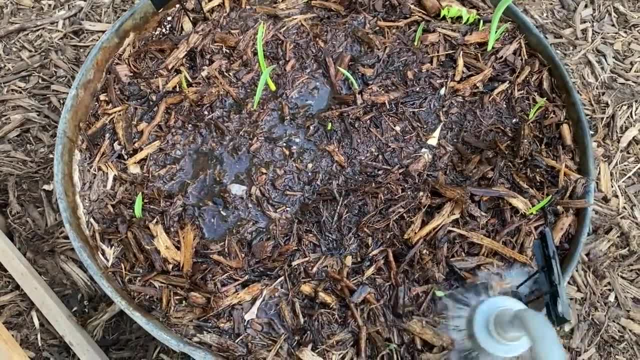 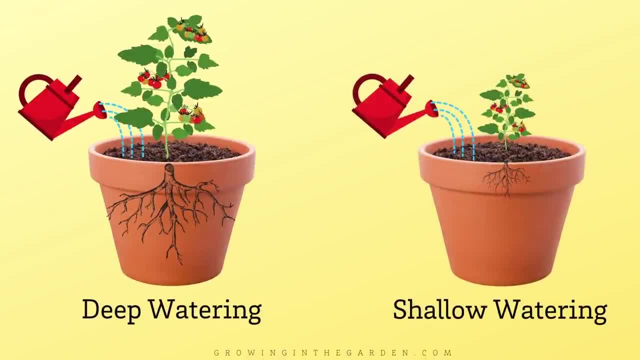 and drench that entire container until you can see water coming out that drain hole. Then you know you have watered that container enough. Deep watering encourages the plant's roots to grow nice and deep, Shallow watering keeps those plants roots right at the surface and they will need 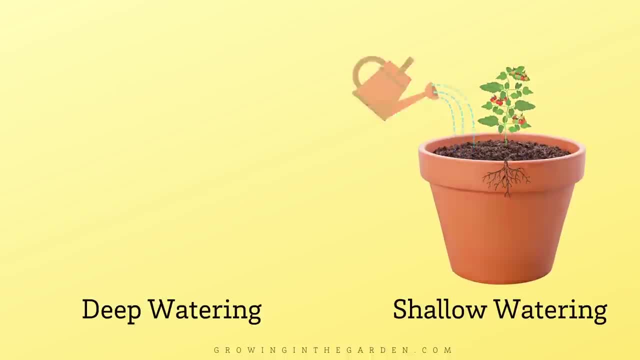 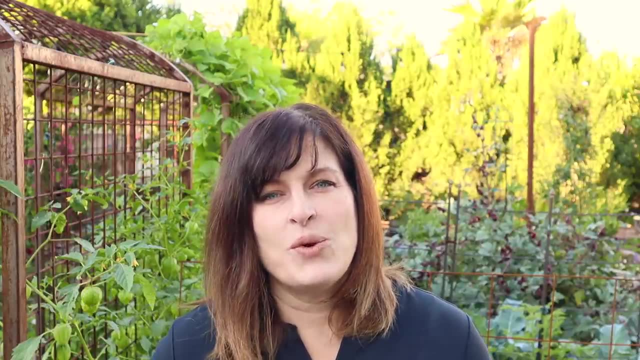 more frequent watering and be more susceptible to stress damage. Another consideration: when you're growing plants in containers, they will need to be fed more often. When the water drains out the whole of the container, it's taking a lot of nutrients with it and we need to add those. 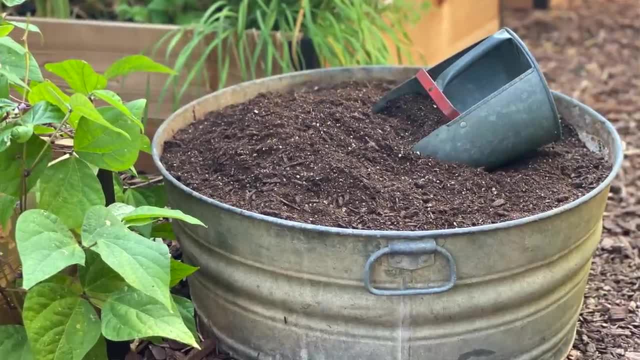 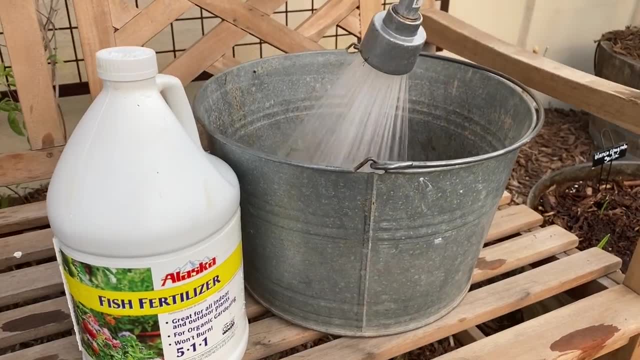 nutrients back in. Compost-rich potting soil will provide some nutrients for the first few weeks and then after that I like to use a water-soluble potting soil. I like to use a water-soluble potting soil that has a lot of nutrients in it. I like to use a water-soluble organic fertilizer like fish emulsion. 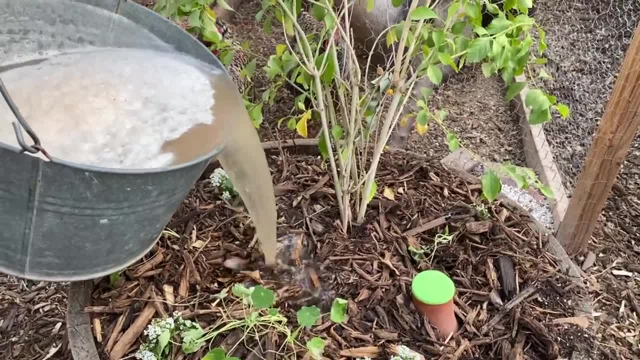 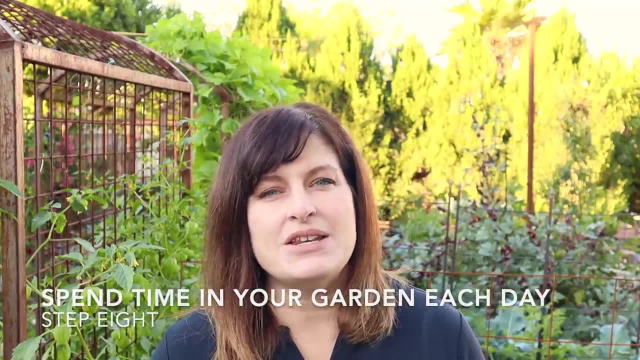 or liquid seaweed, or a combination of both. Follow the dilution instructions and use it as a soil drench on your container plants. It's important to spend some time in your garden every day. Make it a habit to spend a few minutes looking at your plants. Check that your plant's water needs.